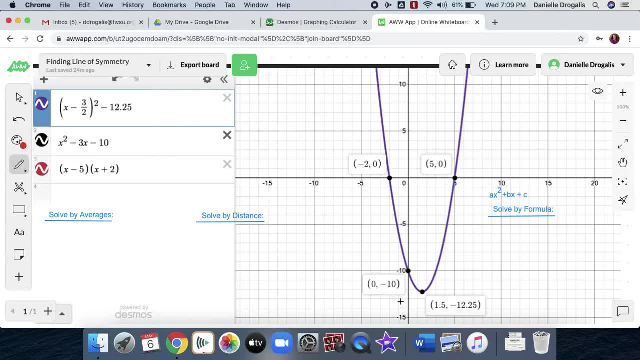 matches the way you think about these math problems. okay, So as we go through, try each one on and then use the method that is maybe the fastest or the most understandable. okay, There's no right or wrong way to do these. You just want to find the one that works for you and gets you. 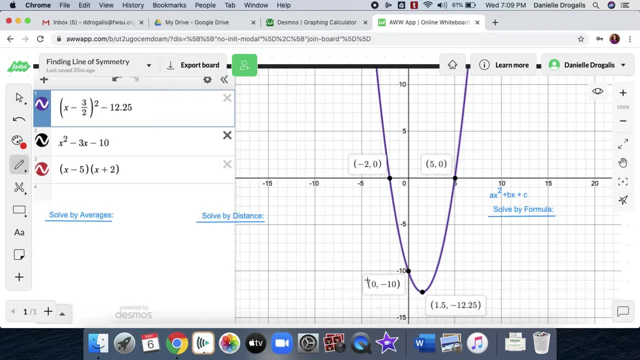 the right answer every time. So the line of symmetry is this idea that if you were to place a mirror somewhere on that parabola, on this curve, that the mirrored image would create the other half of the parabola. okay, So that is the line of symmetry. So let's say we've already. 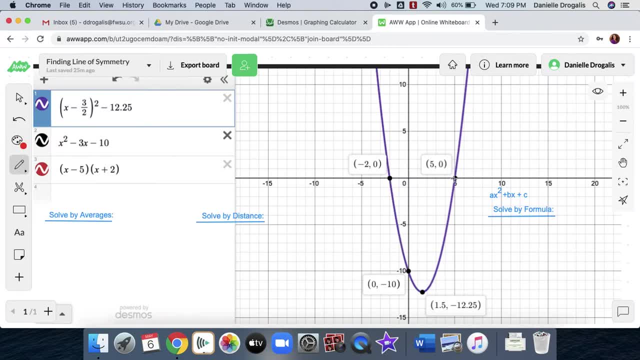 graphed the parabola right And we have the points. but now the question is: what is the line of symmetry? Well, you're going to see that the line of symmetry is the line of symmetry. you're going to use your x-intercepts here, So we have negative 2, 0, and 5, 0,, 5, 0.. And so we're. 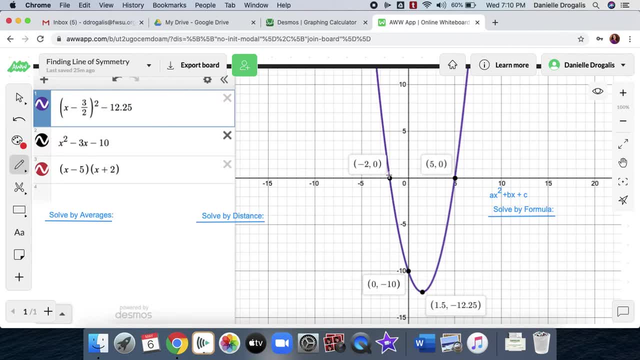 going to use the x-components of both of those, And what we can do is solve by averages, which I will show the work here. So the laws of average say that you add up your quantities, divide by the number of things you added together, and then that is your average. So when you take a look here, 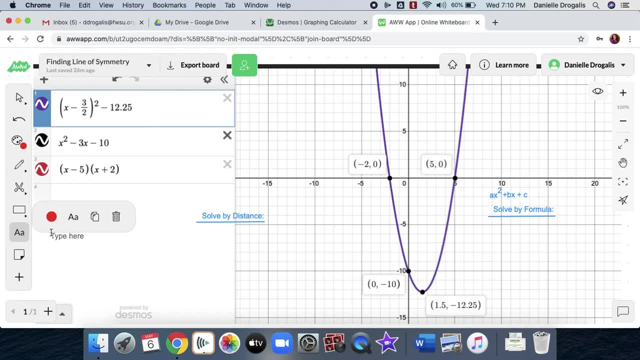 this right here is going to be 5.. So negative 2 plus 5, and we're going to divide that by 2,, okay. Okay, because we had two things we added together, And so negative 5 plus, or sorry, negative 2 plus 5 is going to be a positive. 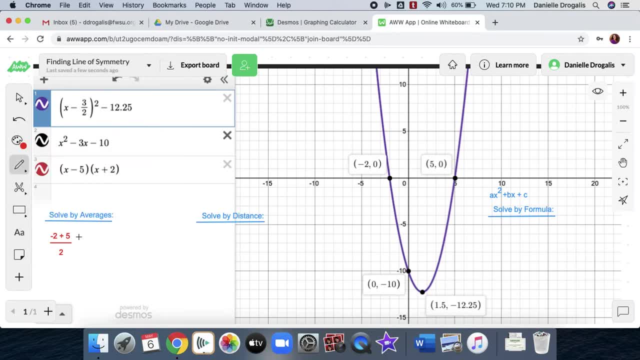 3.. I think, just for efficiency's sake, I'm just going to write it out. So we're going to have a 3, and then, divided by 2,, we're going to get that this is equal to 1.5, or 3.5.. So we're going to. 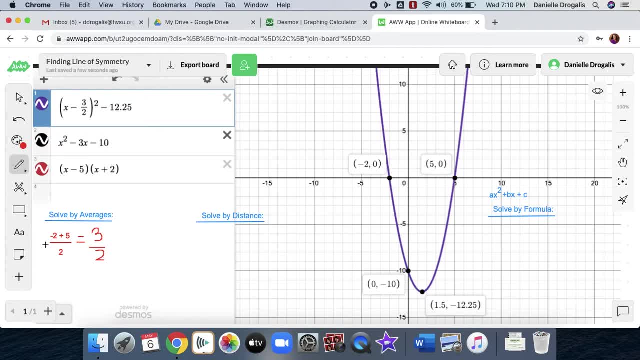 have. this is just as accurate. And so because we're looking for a line, a vertical line, that's an x equals line, And so this becomes x equals 1.5.. And that will be our line of symmetry. And I'm just going to go ahead and show you that line of symmetry on the graph right now. 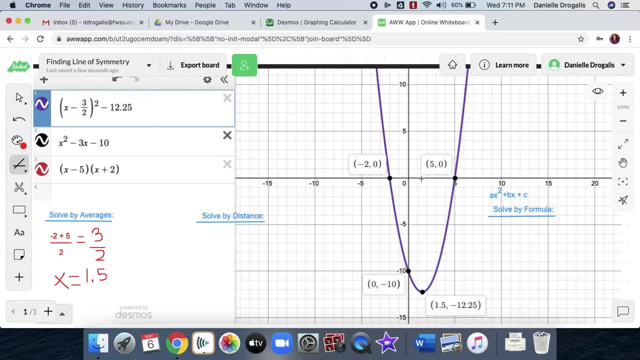 So the line of symmetry- so we go over 1.5- is going to be here And I'll extend it up toward the top also There. So there's our line of symmetry and x equals line. The other way you can do it. 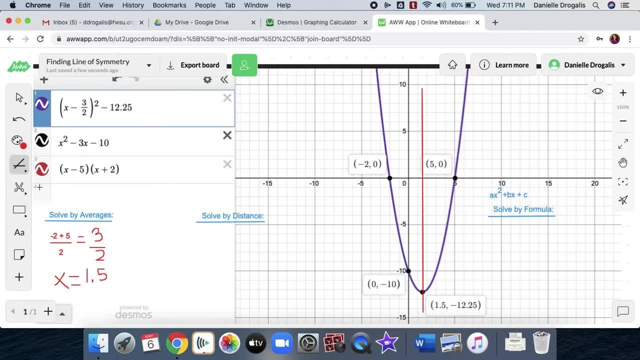 and this is pretty straightforward. I got to say solving by averages is a great way to do it. But maybe you think in a different way, So here's another way. What if you looked at the total distance between these two x-intercepts? So there's two units here and five there, That's. 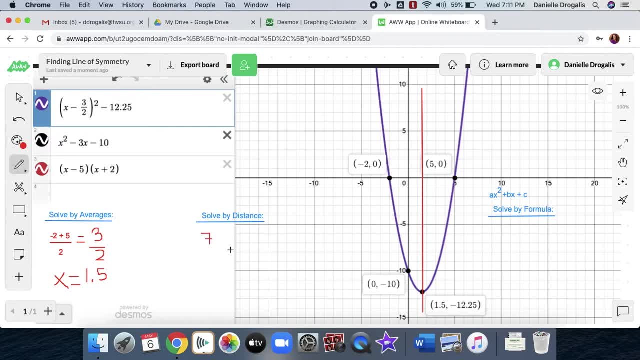 a total of seven. So there's a distance of seven units between the two x-intercepts And you know that the line of symmetry is going to be halfway through there. So we need half of that. So that'll get us a 3.5.. Now the difference here is that this output is not the axis of symmetry. 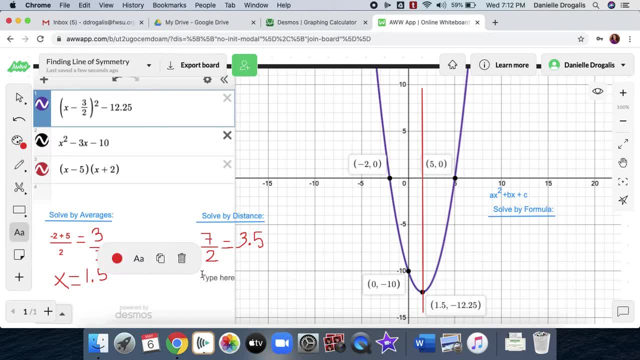 but rather it's the counting distance you need to go. So this is the distance that you count from each intercept, from each x-intercept toward the other one. So, for example, if you're at negative two, you got, you have to count. 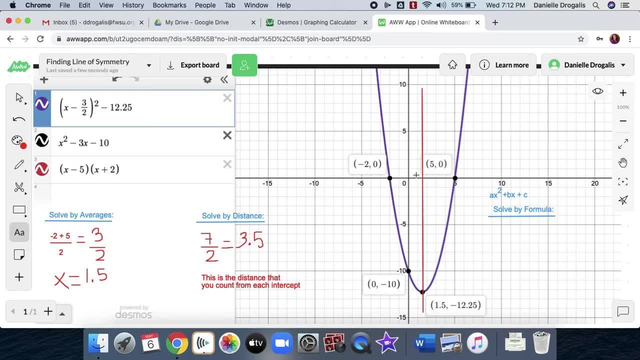 you have to count three and a half units to the right. So one, two, three and a half and you land at 1.5.. If you are at five, you count three and a half units toward the other point. you go one, two, three and a half and right away you land at 1.5.. So this is a different way. 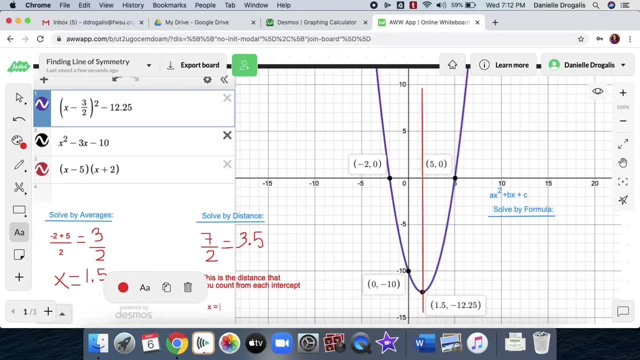 to think about how the x or the line of symmetry is. whoops, there we go: 1.5.. It's another way to get to that. So just be careful with this one. It's great If you like this one. just be careful that the output 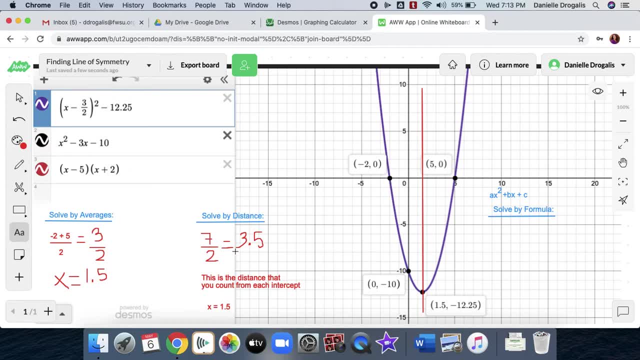 is not going to be your actual value of your line of symmetry. It's the amount you need to count away from that point toward the other one to land at the right location. Okay, So now this last one has to do with the formulas. Now, some people really think in formulas, but I got to caution. 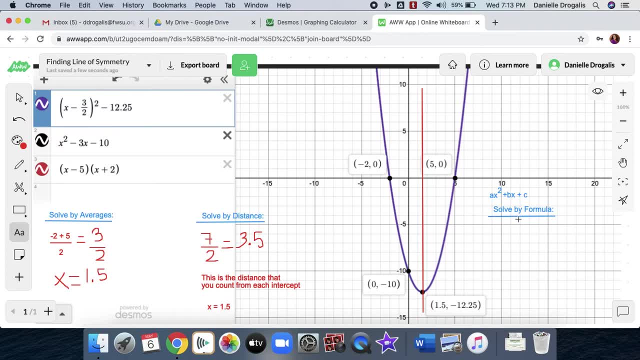 you, depending on how you think about it, like for me, for formulas, they tend to be more accurate, So I'm going to be more accurate with this one. So I'm going to be pretty mindless exercises where I just gather information, I plug it in and compute it. 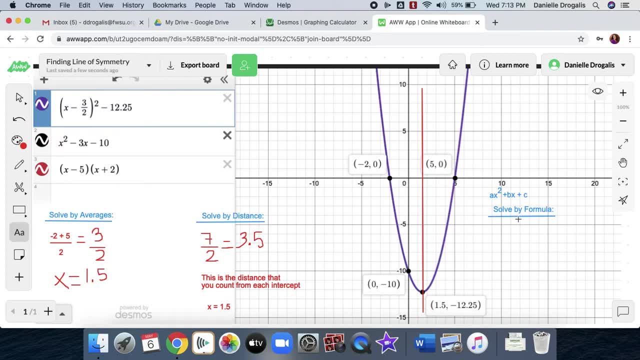 but I don't really have like a full understanding of its importance or value all the time. I just know I can follow a series of steps to get the answer. So don't choose this one if you see it as an easy way out. right? You don't want to minimize your chance to understand this stuff. 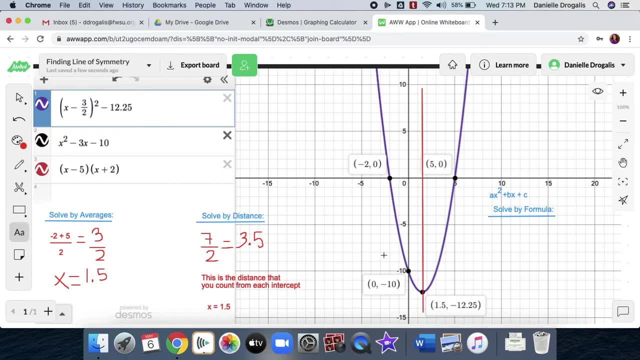 like truly understand it. but maybe you think in formulas, right? So this means that you have your typical trinomial formula. This is the one you would use if you only had this equation. Okay, So if you only had that equation or the other two, and you could create this standard form from the other two? 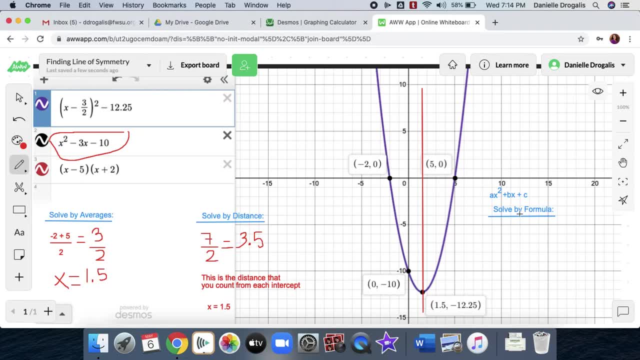 equations, then you could do this work. So if you had no graph visible to you and you only had an algebraic approach, this is what you would do. So the formula here is that the line of symmetry is equal to the opposite of what you would do if you only had this equation. So if you only had this, 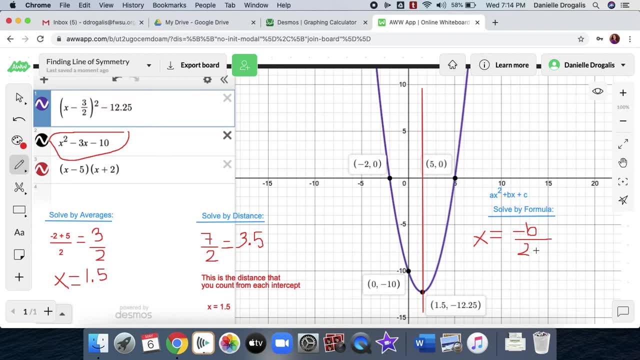 equation, then you would do this work. So if you only had this equation, then you would do this work. whatever b is over two times whatever a is in the formula. So this is your generic formula of a quadratic. We also call this a trinomial, And so if you look over here, this is that equation in 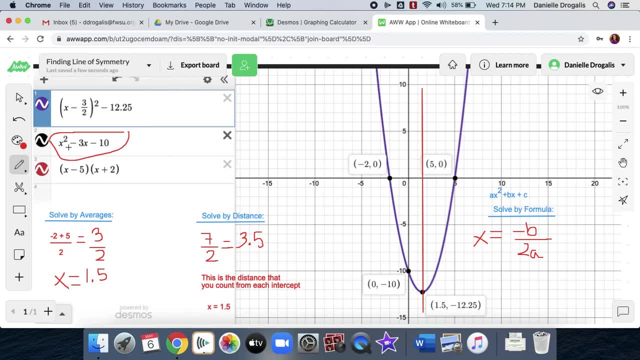 this is the form that you'd want. This is your trinomial, your standard form. that will help you out here. So the a term is one, the b term is a negative three- make sure you take the sign with it- And your c term is a negative 10.. This formula is just concerned with the 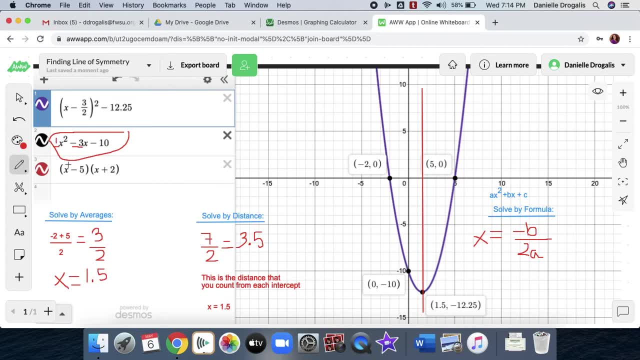 B and the A and the A. hiding in there is a one, So then you're just substituting in. like I said, that's the tendency of a formula, but it can be a risk, right? So don't shortchange yourself with. 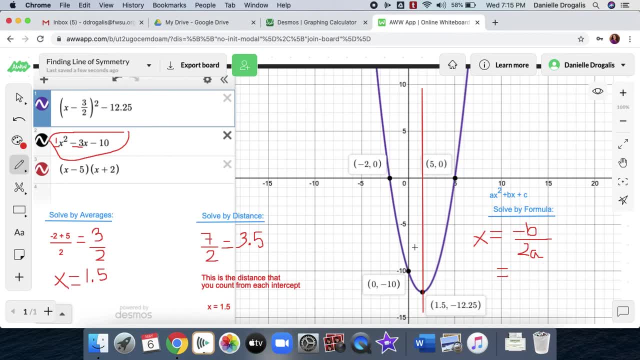 your learning and don't do the formula if you don't understand it. So negative or the opposite of B. So B was negative three. So notice I have two signs by having parentheses when I substitute will always help me navigate a double sign when I'm supposed to encounter it Otherwise. 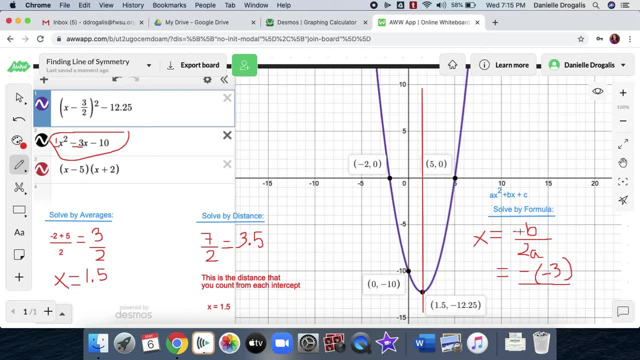 the common mistake here is people will just write negative three because they write negative and then the three and they think that the negative three, that was B, has taken care of the negative in the formula as well, which it has not. So if you're inserting a negative B,